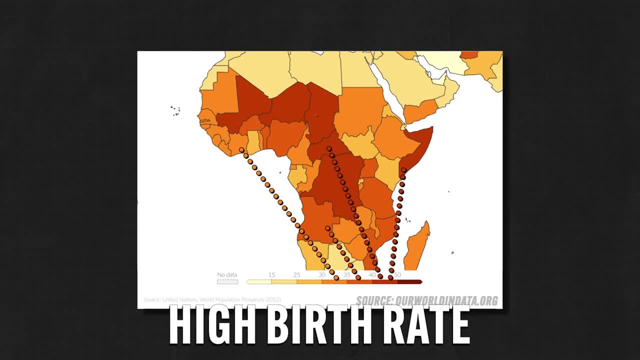 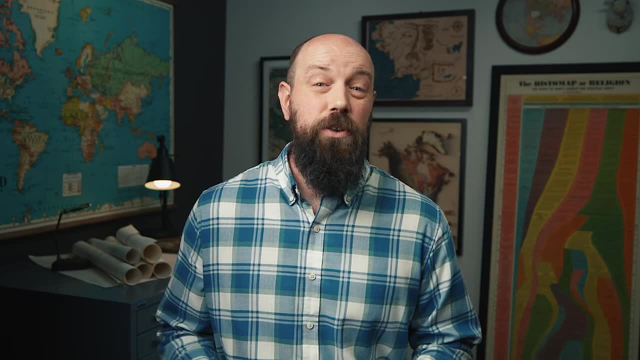 And then down here in Sub-Saharan Africa, several places have a high birth rate, which is a CBR greater than 30. So if Heimville's CBR is a hundred, well you know we got babies for days. Anyway, here's where I tell you that the crude birth rate is crude. 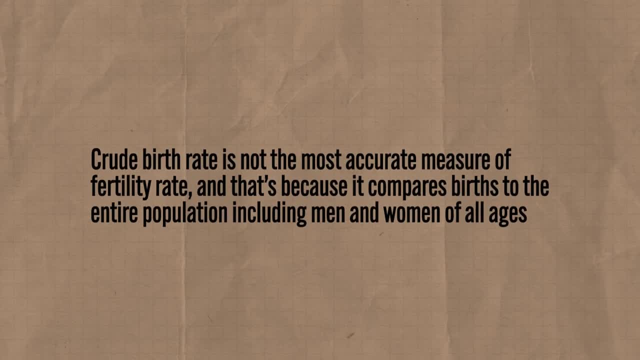 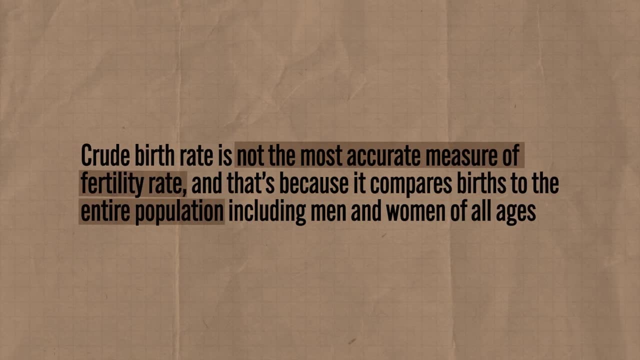 not because it indiscriminately drops colorful language at family dinners. It's crude because it's not the most accurate measure of fertility rates, and that's because it compares births to the entire population, including men and women of all ages. So is there a more accurate measure of fertility rates? 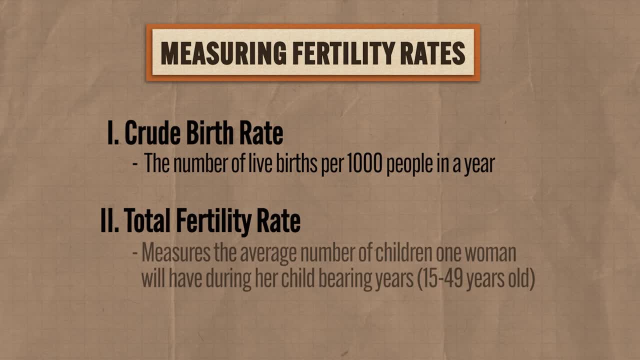 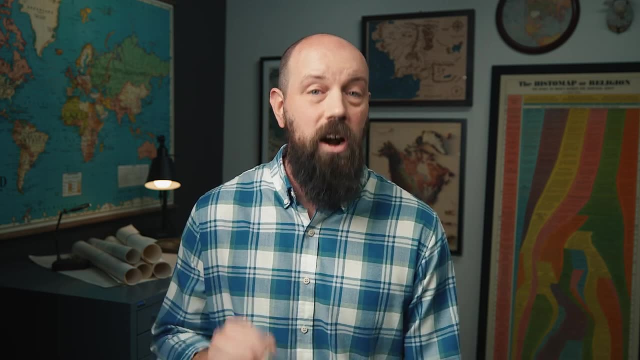 You know, there is, and it's called total fertility rate, which measures the average number of children one woman will have during her childbearing years, which is to say 15 to 49. And the reason total fertility rate, or TFR, is a more accurate measurement is because 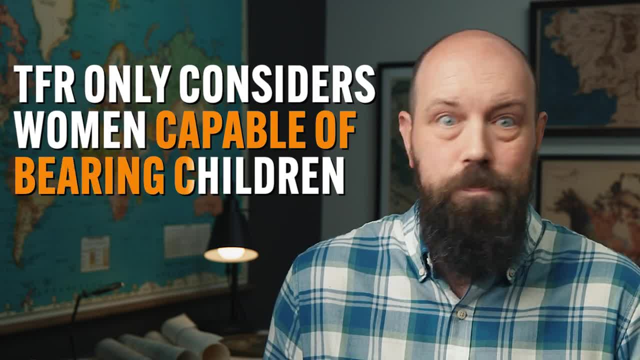 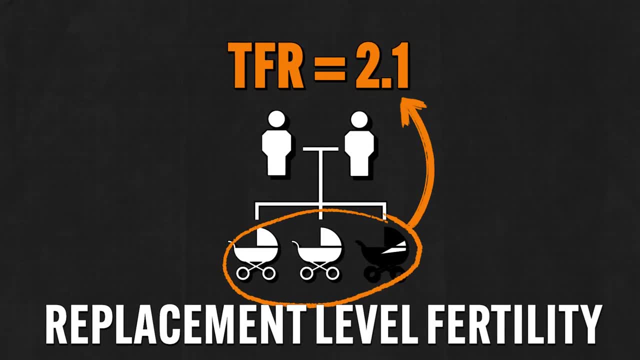 it only considers the part of the population that is capable of, you know, bearing children. Okay now, a TFR of 2.1 is what we call replacement level fertility, because that's the number of babies that are required to replace the two people that had them. 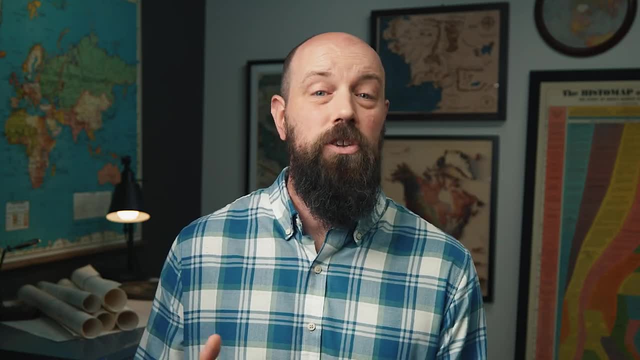 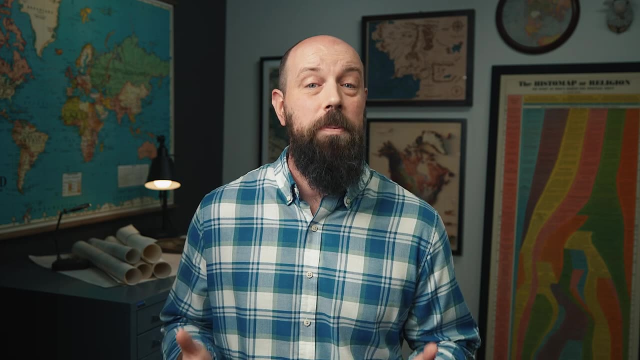 Now, not surprisingly, these numbers correlate pretty well with what we saw in the spatial arrangement of the crude birth rate. Europe's TFR averages to about 1.6, which, if you recall the replacement fertility level, means that Europe's population is not going. 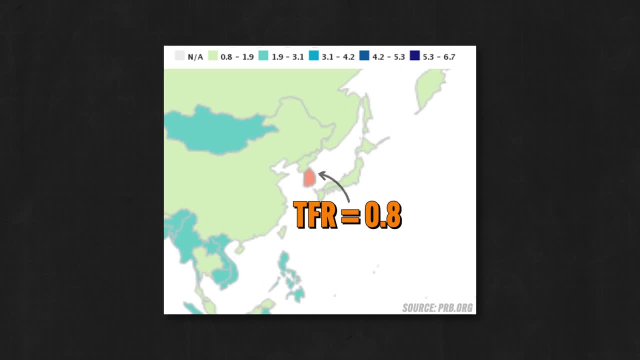 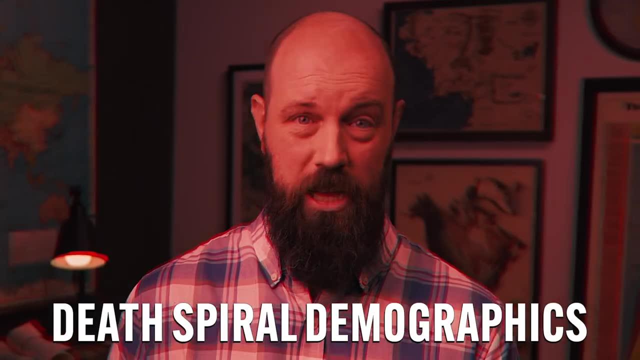 to replace itself and therefore it is declining. Other places like South Korea and Puerto Rico have even lower TFR numbers and they have entered the shiny, happy world geographers like to call death spiral demographics, But Sub-Saharan Africa's TFR is around 4.6, which again babies for days. 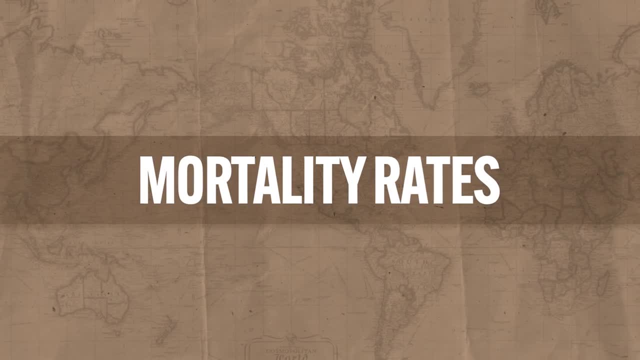 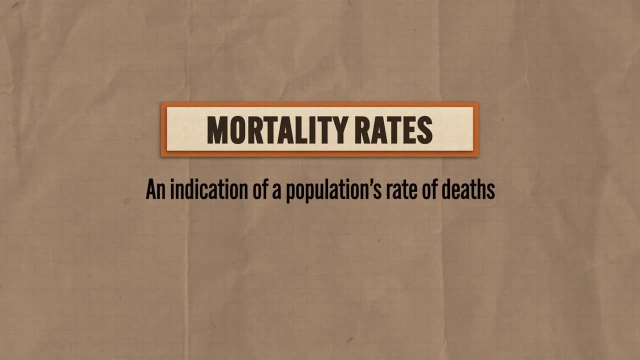 Okay. so fertility rates help geographers measure population growth or decline. but on the other end of the demographic spectrum, we've got another way to measure it, and that's called mortality rates, And that's just an indication of a population's rate of deaths. 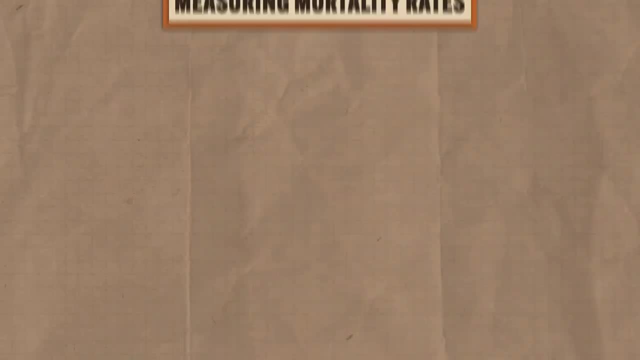 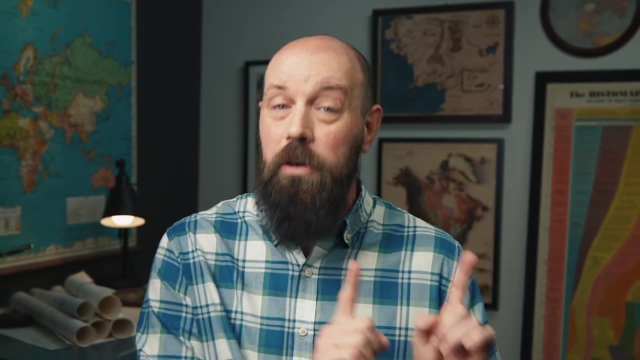 And wouldn't you know it, there are two ways to measure mortality as well. First is the crude death rate, which is the number of deaths per thousand people. Now, despite its crudeness, CDR is a more accurate measure of death than crude birth rate is a. 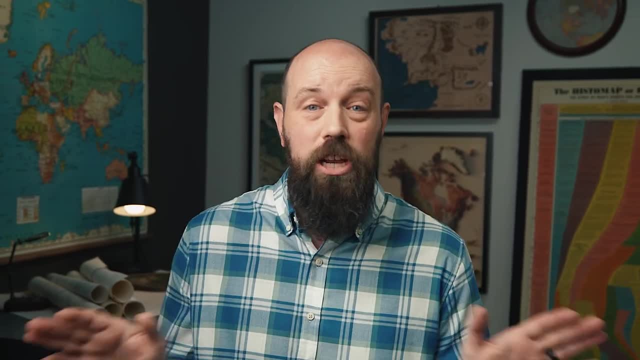 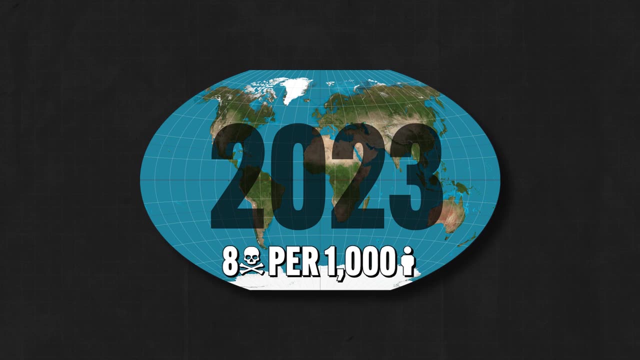 measure of fertility and that's because, you know, last time I checked, regardless of gender or income or education or whatever, everybody dies. Sorry to be a bummer, but it's true. So currently, the global crude death rate is about 8 per thousand people. 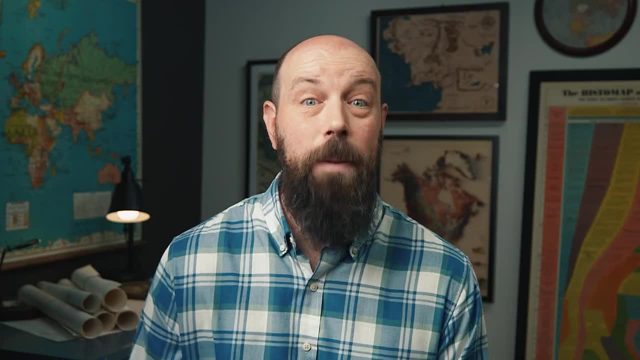 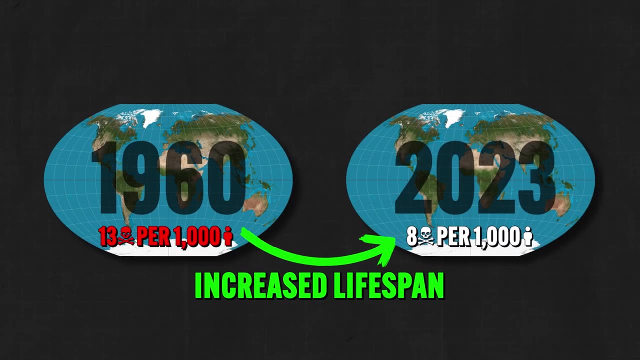 But back in 1960, it was 13 per thousand. So what does that mean? People are living shorter lives now. No, Get back in your cabinet and keep studying. The decrease in CDR means people are living longer lives now. So what does that mean? People are living shorter lives now. 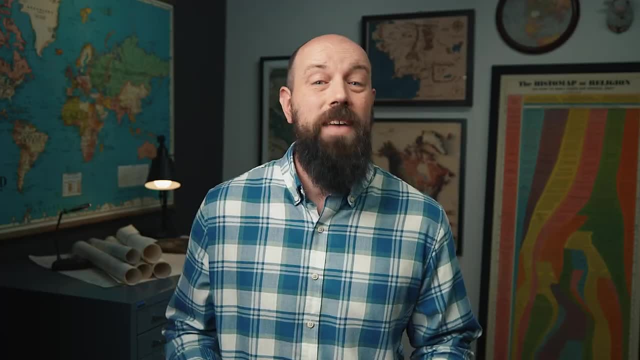 No, Get back in your cabinet and keep studying. The decrease in CDR means people are living longer lives now. But why would that? be Well, in general, people have access to better nutrition, better medicines, clean water etc. And that means global life expectancy has increased. 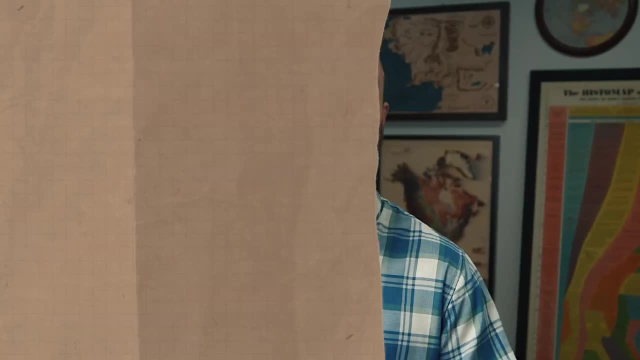 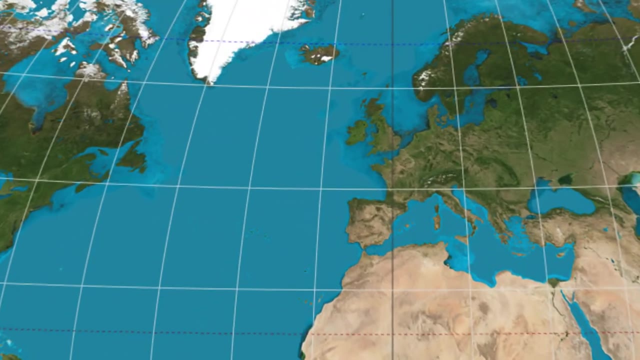 But here's where I tell you that, depending on the scale we're considering, that generalization falls apart At a national and regional scale. life expectancies vary according to how wealthy a nation is Like. in some developed nations, the life expectancy is 80 years, while in many 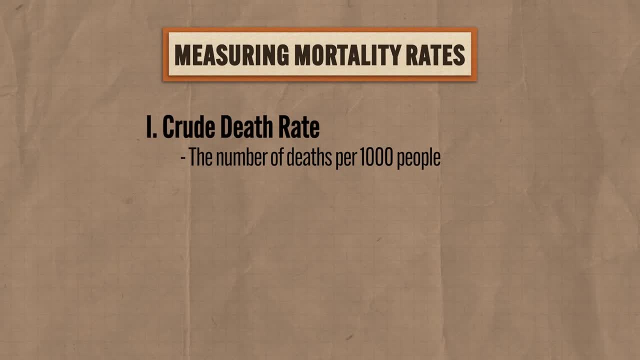 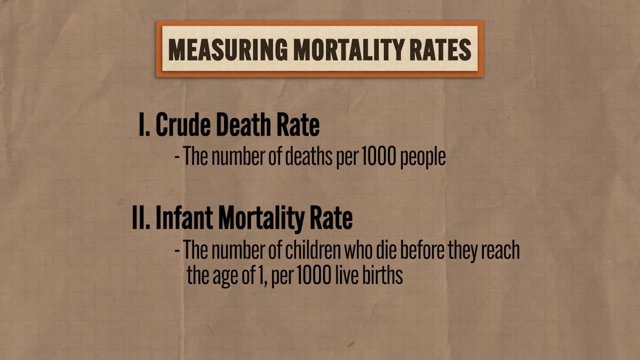 developing nations, it's more like 50 years. Okay now, the second measure of mortality rates you need to know is the infant mortality rate, which is the number of children who die before they reach the age of one per 1,000 live births. And what the IMR is really good at showing is a country's 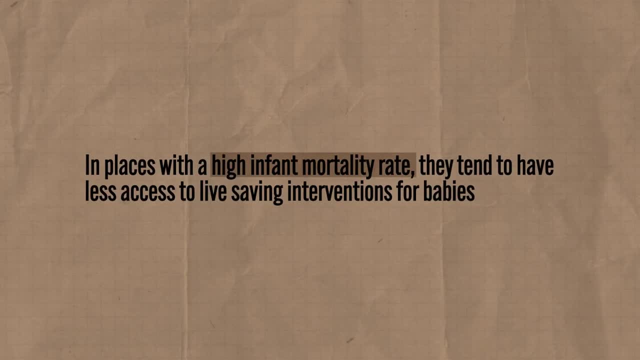 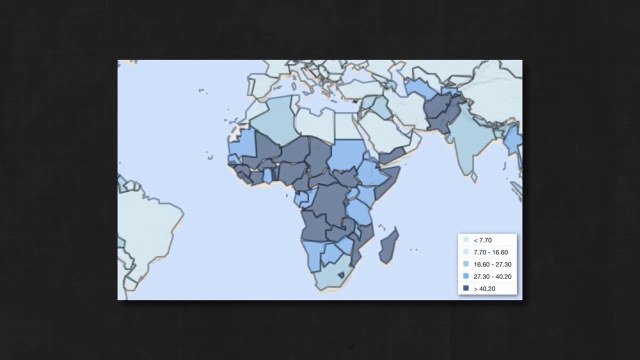 access to healthcare. For example, in places with a high infant mortality rate they tend to have less access to life-saving interventions for babies. So you can see here that a lot of the world has low infant mortality rates, but in Sub-Saharan Africa the rates are pretty high. 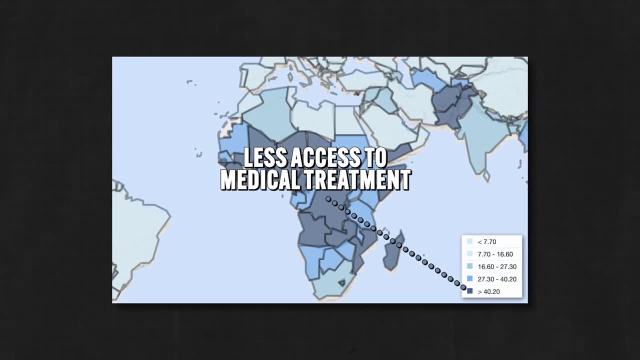 which would indicate less access to medical procedures for infants and mothers. Now, migration is also a major factor in population growth and decline, but we're going to consider that in depth later in Unit 2 videos, so we're just going to leave it. 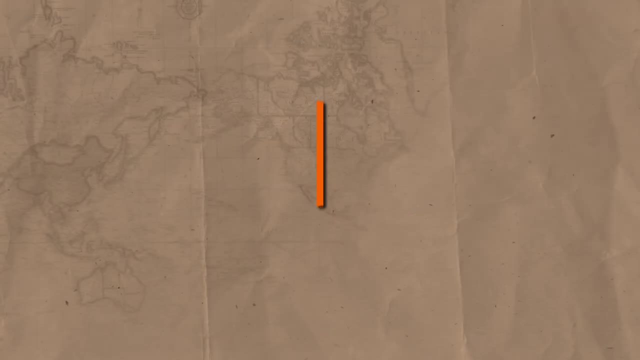 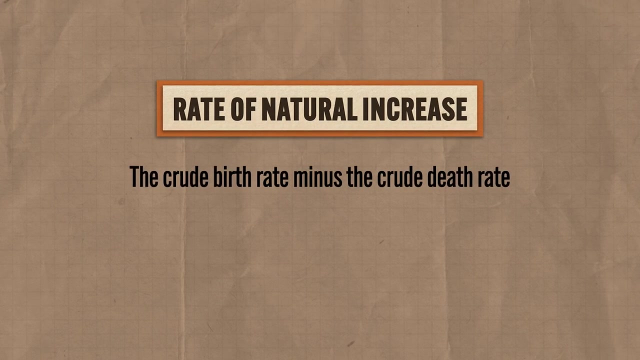 there for now. Okay, now let's pull all of this together. When geographers want to explain the reasons for population growth and decline, they use a measurement called the rate of natural increase, which is the crude birth rate minus the crude death rate, And this is relatively. 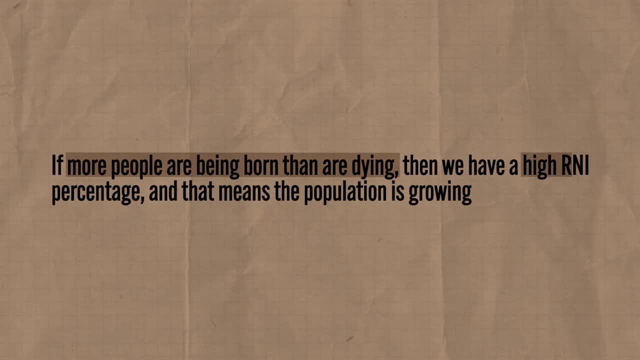 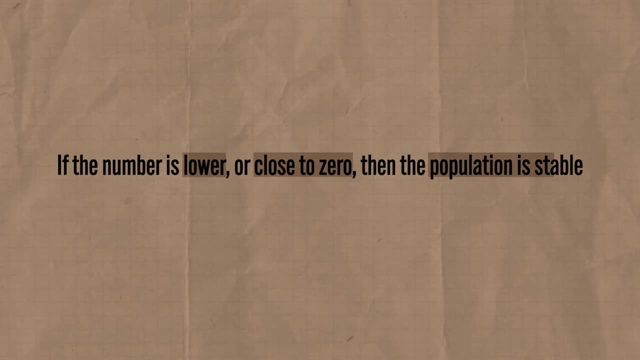 simple to understand. If more people are being born than are dying, then we have a high RNI percentage and that means the population is growing, like we saw in Sub-Saharan Africa. But if the number is lower or close to zero, then the population is stable, like it is in the United. 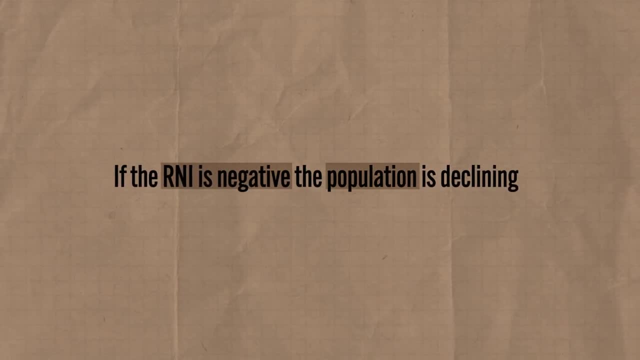 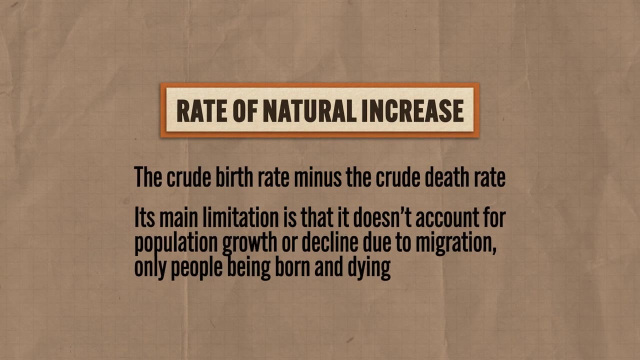 States. But if the RNI is negative, like in Germany, well, the population is declining. However, one note on the rate of natural increase. Its main limitation is that it doesn't account for population growth or decline due to migration, only people being born or dying. 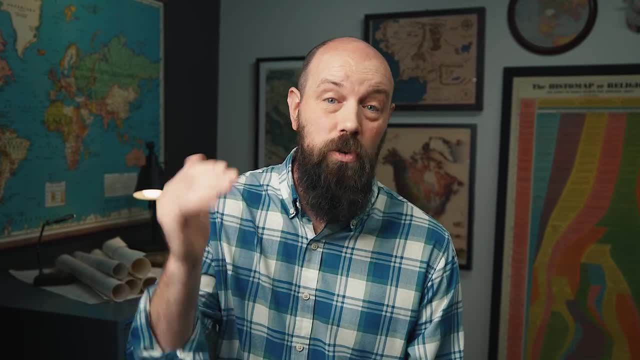 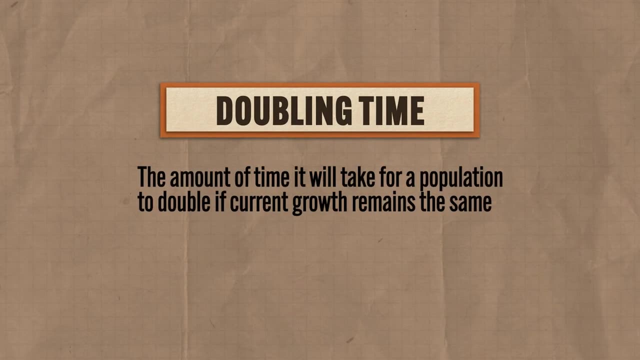 Like a country might have a negative RNI but still experience population growth if lots of immigrants are coming in. Okay, now a related measure for population is known as doubling time, which is the amount of time it will take for a population to double if current growth remains. 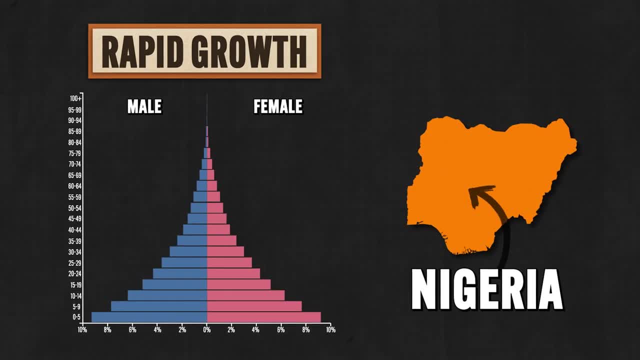 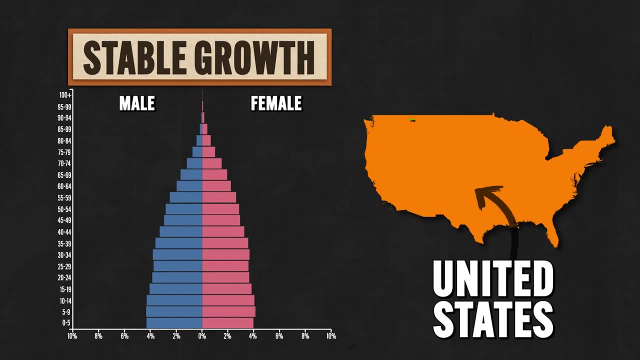 the same A country like Nigeria is experiencing explosive population growth at around 2.6% per year, and that means the doubling time will be about 27 years. But in a slower growth country like the United States, at about 0.3% per year, the doubling time is going to be: